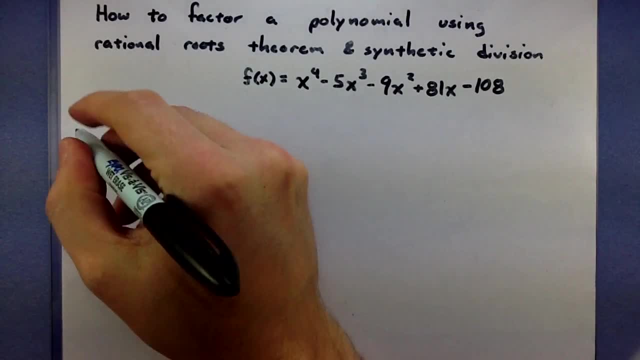 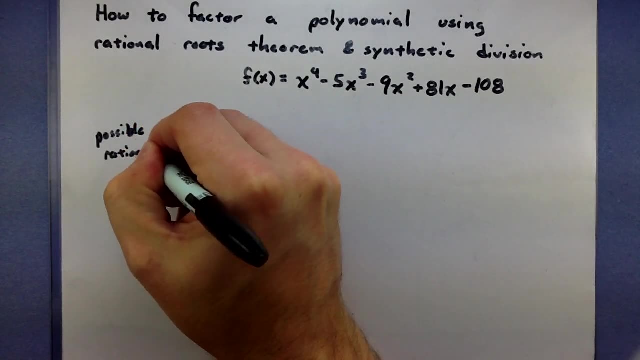 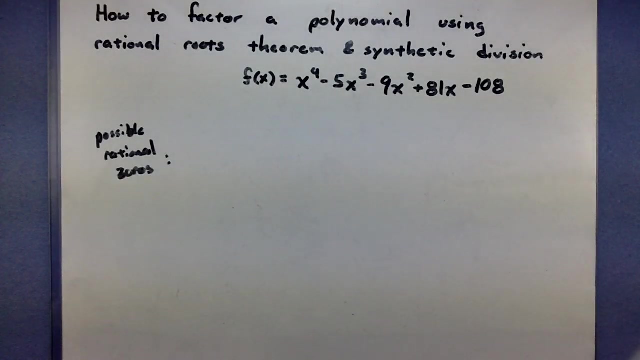 is basically a list of possible zeroes. So to come up with this list of possible Rational, you want to take your factors of the last term- this is the 108, and divide it by the factors of the first term. I like to call these the p over q. Okay, 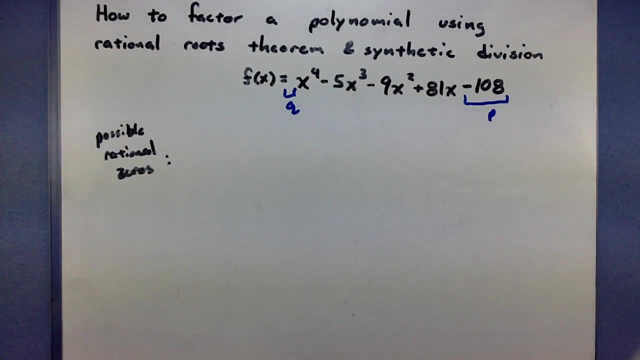 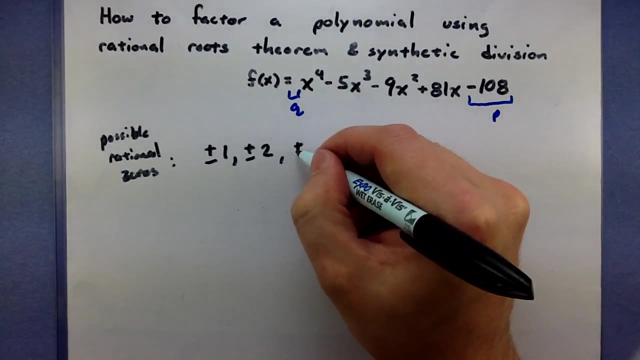 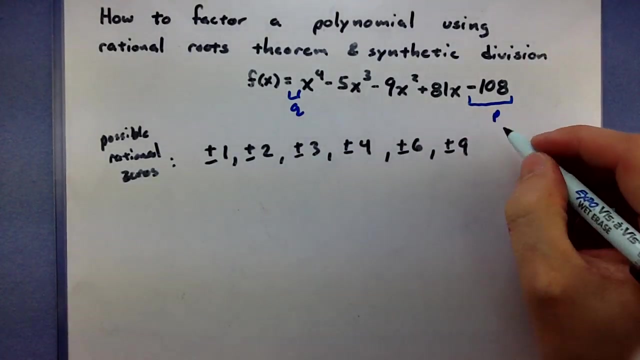 So let's list out all the factors of 108, and they're going to all be divided by 1.. I have basically plus minus 1, plus minus 2, I got 3, 4,, 6, 9,, 12, 18. 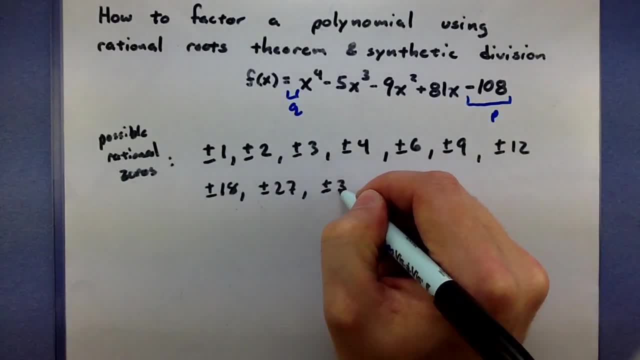 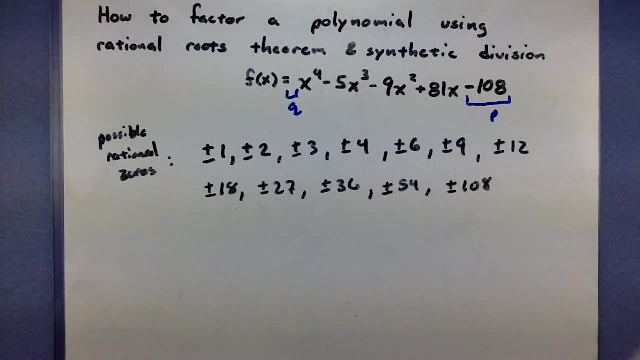 27,, 36, 54 and 108.. Wow, So I have quite a bit of possible rational zeros that I might have in my polynomial and basically we have to test these out one at a time. Now, since I do have so many I kind of want to use. 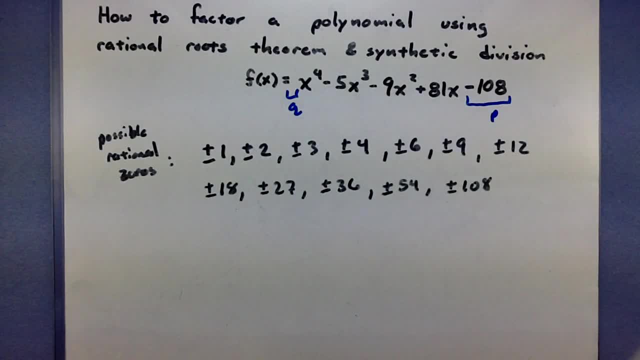 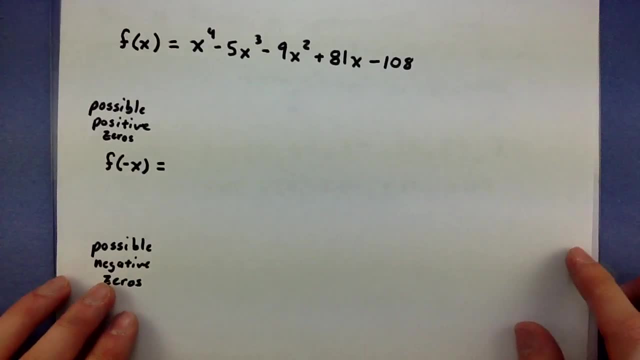 Descartes' rule of sign here, so I can see how many I can expect will probably be positive and how many are going to be negative. Let's go ahead and take a look at that process So to get an idea of the possible positive zeros I might have. 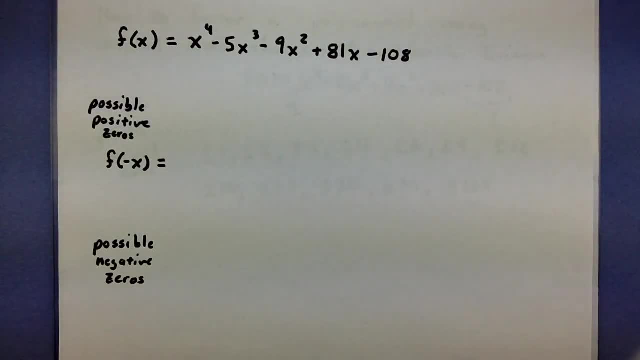 Descartes' rule of sign says that I can count the sign changes in the polynomial and get an idea. So here's that polynomial. Let's see how many times it changes signs. So it goes from positive to negative and it goes from negative. 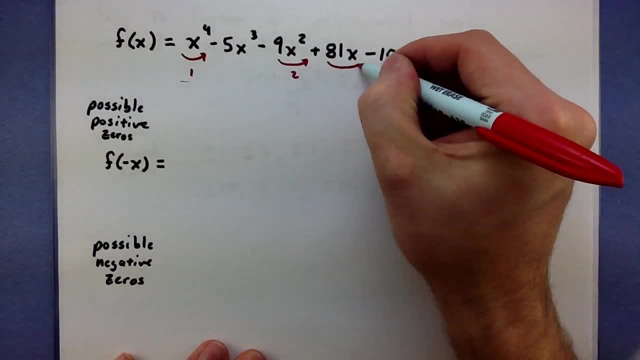 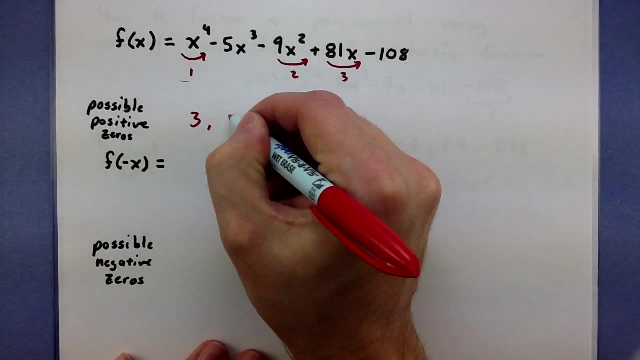 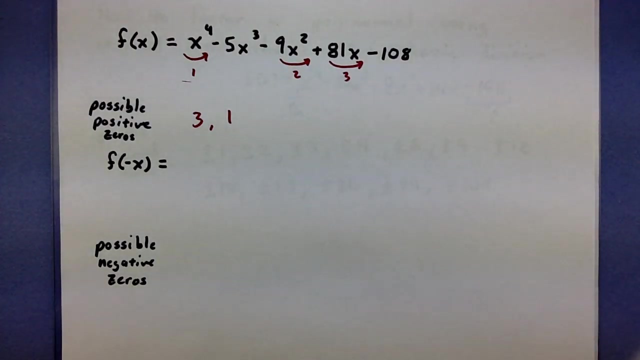 to positive And then positive to negative. So, in terms of how many possible positive zeros could I have? well, I could have 3, or I could have 1.. Okay, not too bad. To figure out the possible negative zeros, we look at f of negative x. 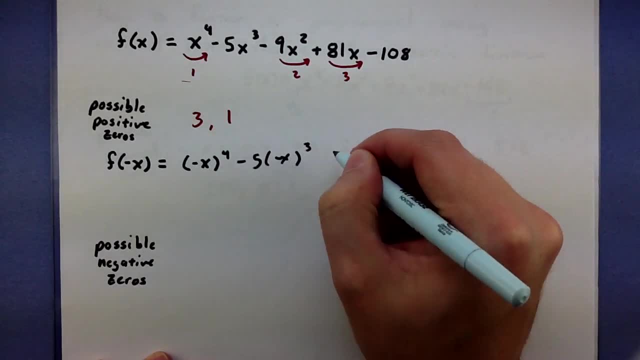 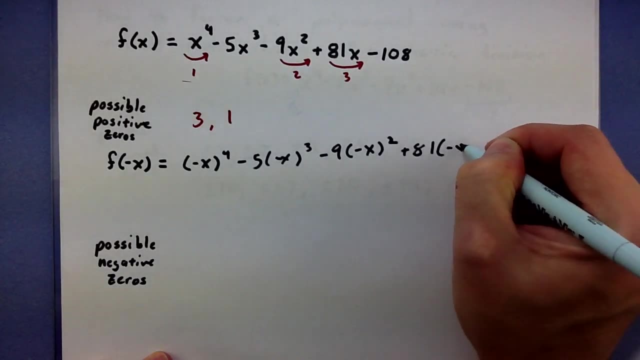 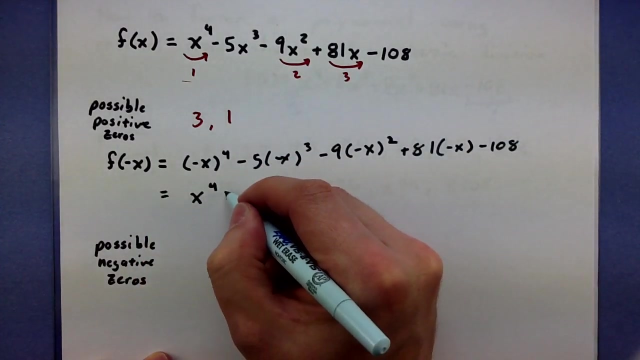 So I put in a negative x for all of my x's, then we'll simplify this and then count the sign changes one more time. Let's see this would be x to the fourth. Let's see minus x to the third and there's already another minus sign, so 5x to the third. 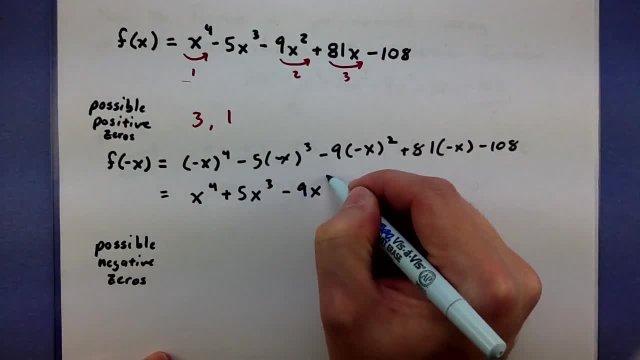 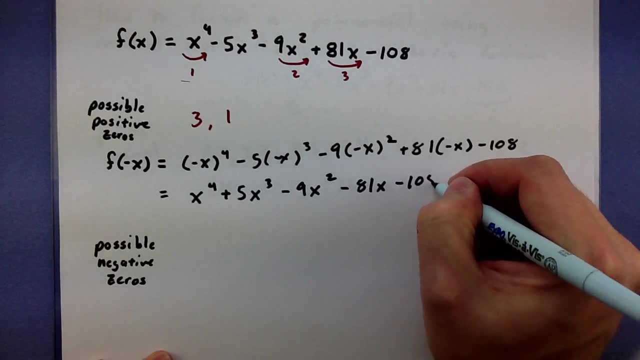 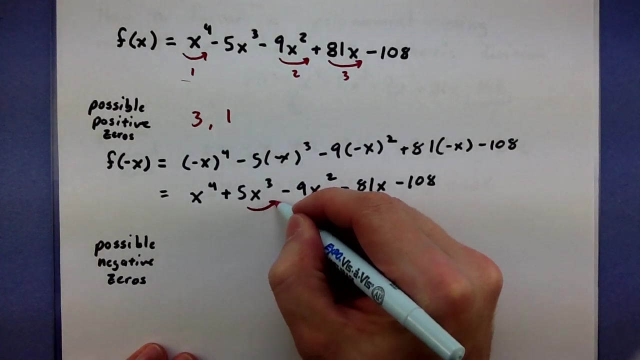 Let's see: minus 9x squared, Minus 81x, Minus 108.. Perfect. So as I look through this, it looks like that we only have one sign change here, So there's probably only one possible negative zero. 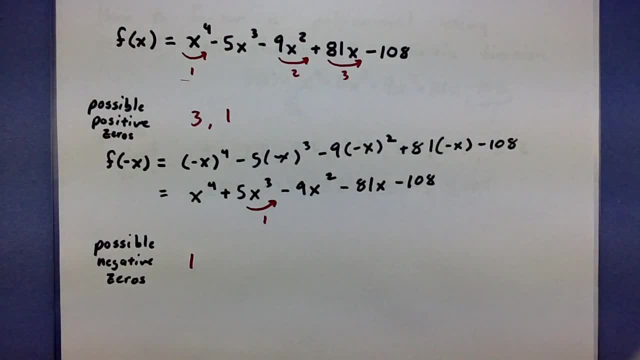 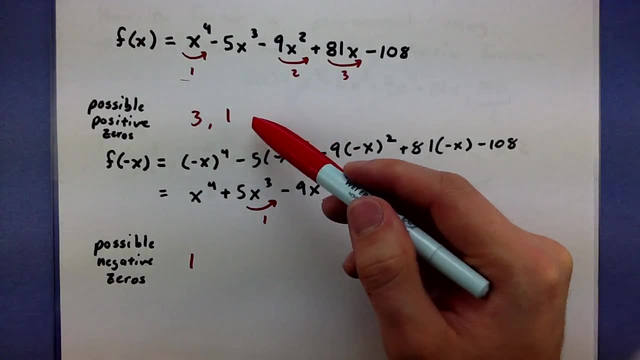 Now remember that, since this is a fourth degree polynomial, I'm looking for four total. So what these possible things tell me is that I could have three that are positive and one negative, or I could have one positive, one negative and two complex. 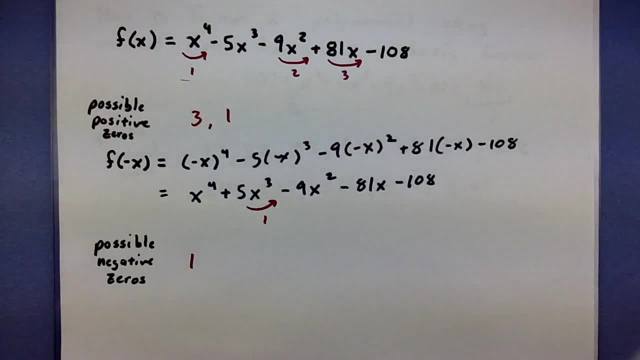 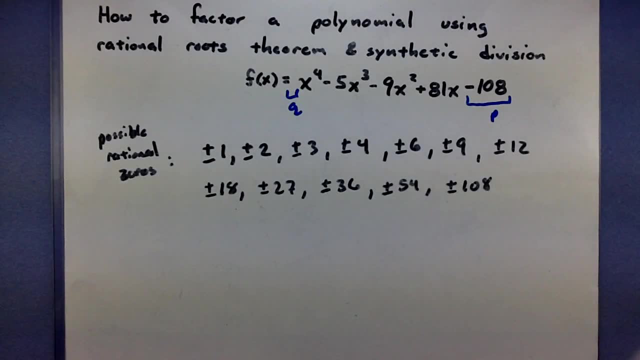 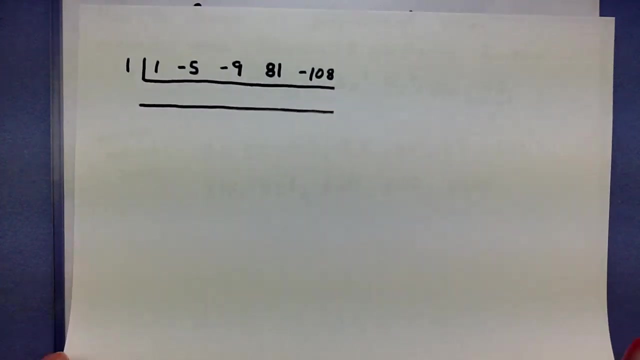 Let's go ahead and set that information off to the side and see if we can start testing out some of these zeros one at a time. So with so many zeros to test, usually I start off with the smaller guys first. Synthetic division is definitely the way to go here because it's the fastest. 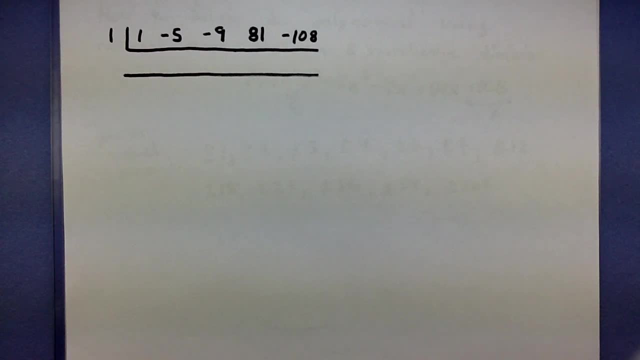 way to test out a zero. So what we're going to do is basically take these guys one at a time In synthetic division. we take the one, drop it down just as it is, We multiply, Then we add, Multiply, Add, Multiply. 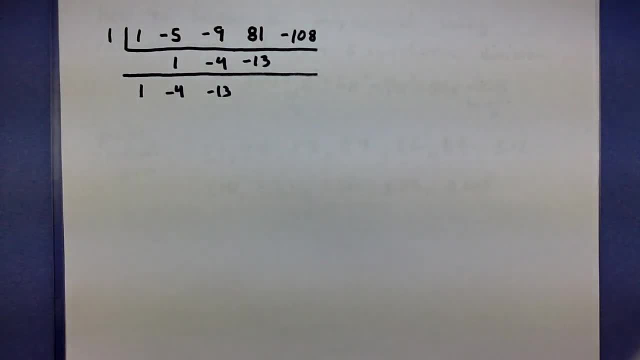 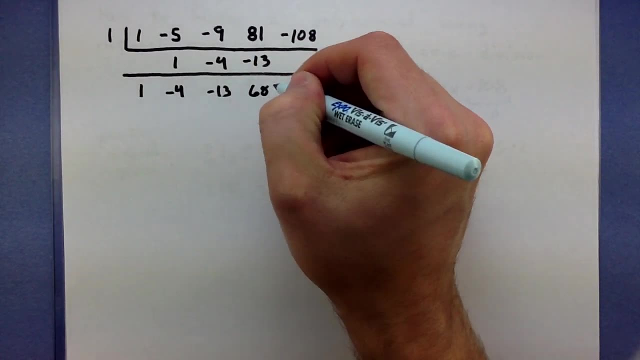 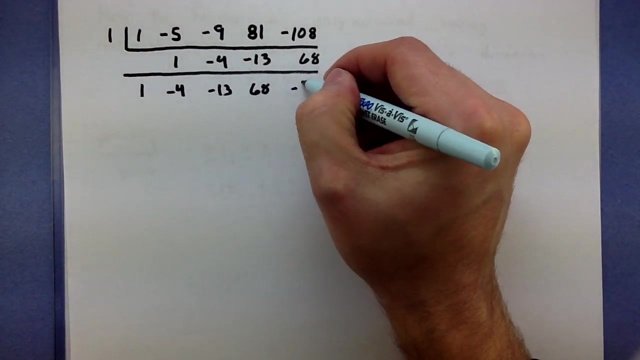 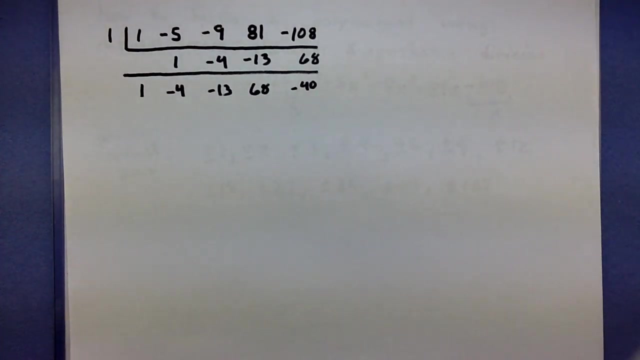 See, now I need to add these two together Looks like a 68. Multiply And this will give me a negative 40. Now what I'm doing every time I test out one of these zeros is: you always want to check out your remainder to see if you get a zero remainder. 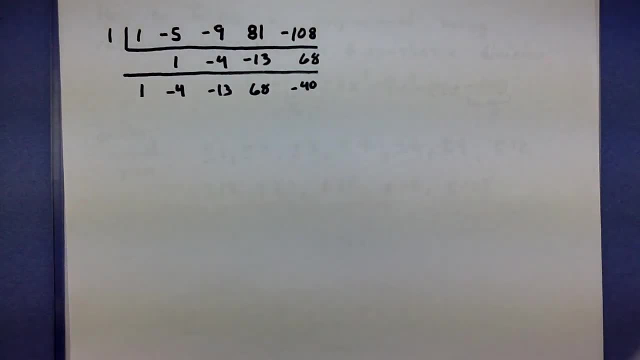 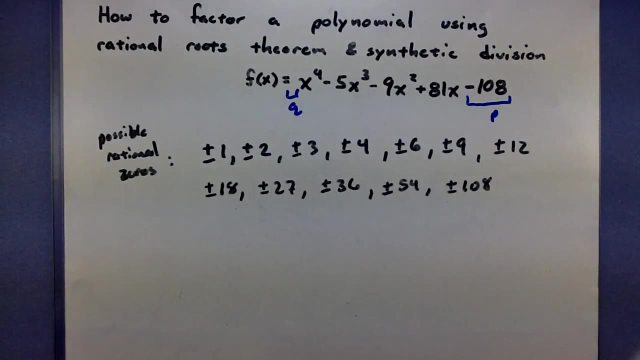 If you do, you know you found a zero In this case, where we got a negative 40, I know it's not one of our zeros, So then you can go back to your list and say, alright, that positive one did not work. 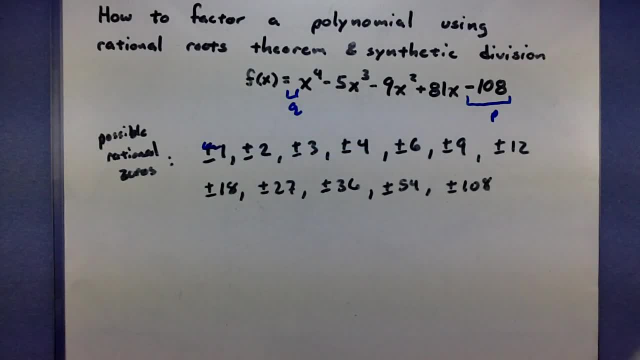 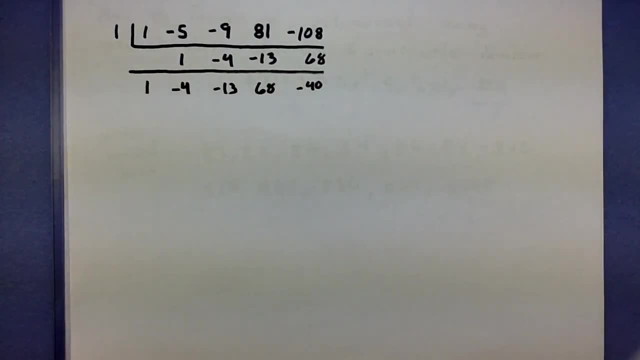 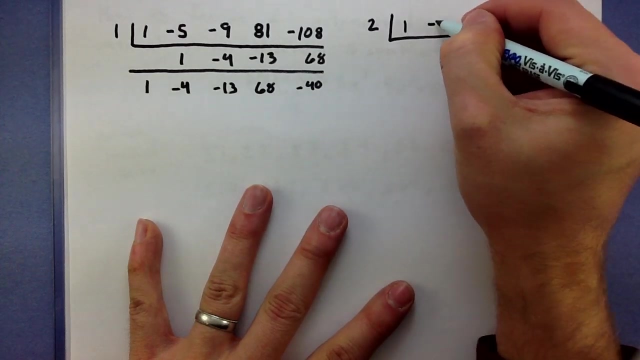 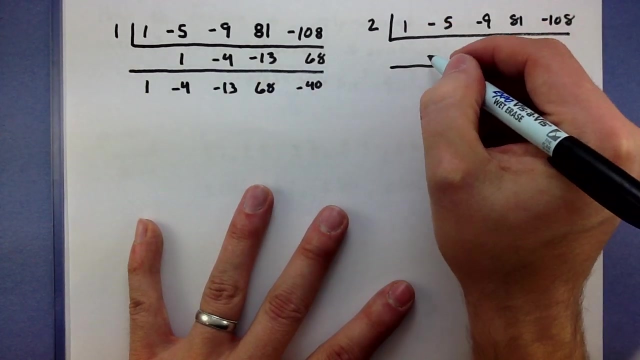 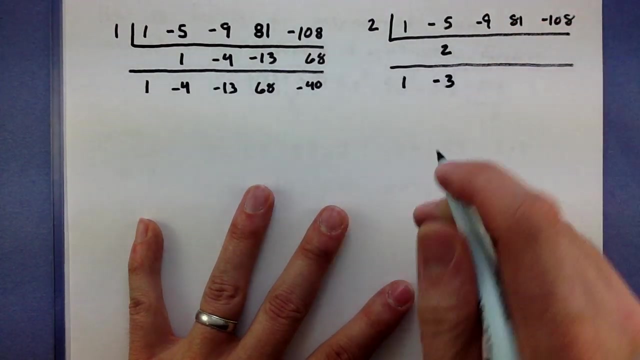 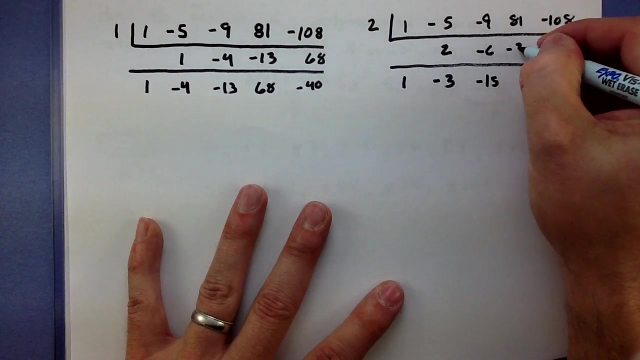 Let's cross it off and test something else. Well, since that one didn't work, I'm going to go on and try and use a two. Alright, so bring down the one. Multiply, Add, Multiply, Multiply, Add, Multiply. 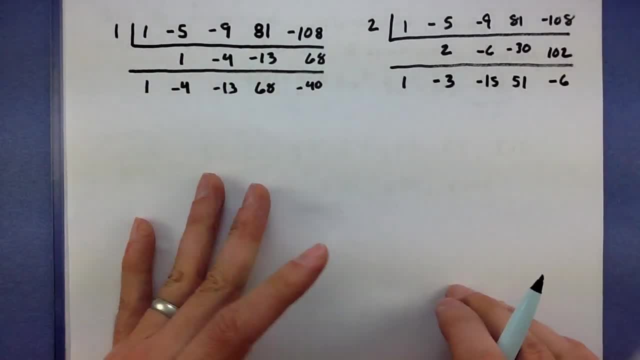 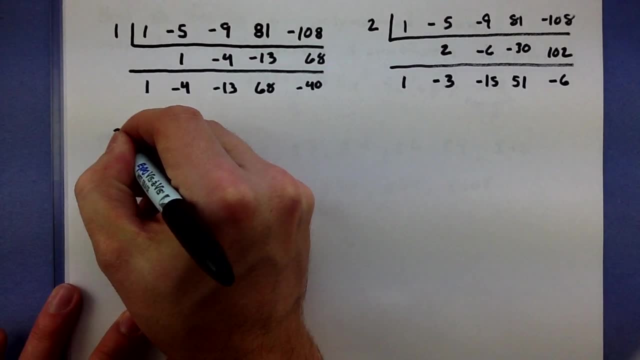 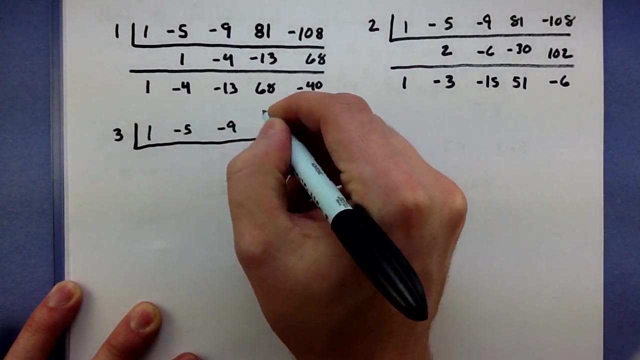 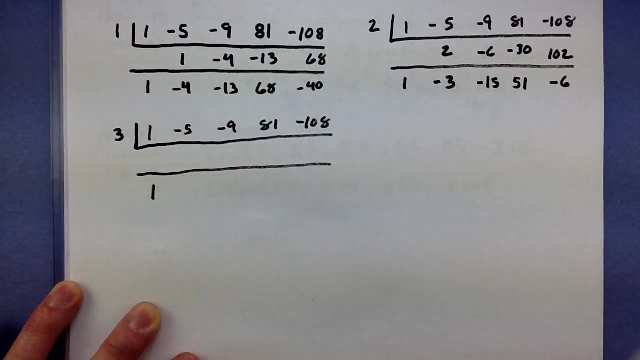 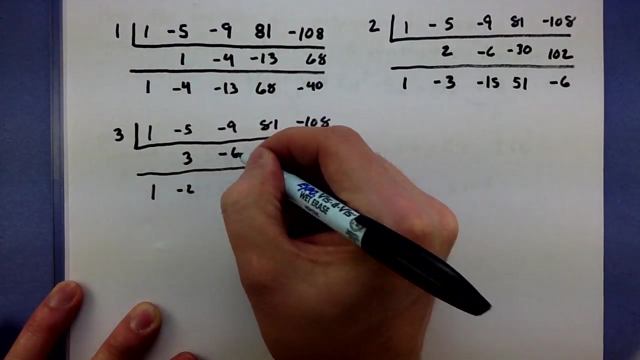 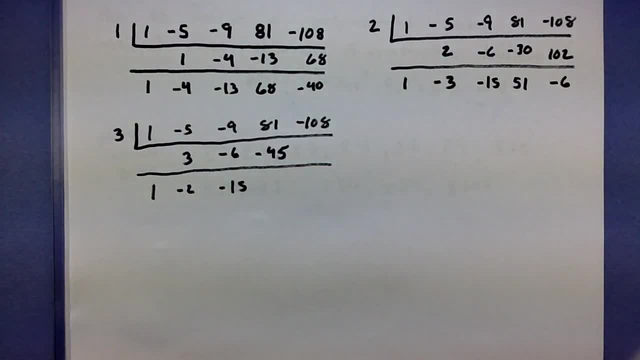 Negative 45. There we go, Add these two together, Multiply And add Hey, what do you know? So it looks like three is definitely one of our zeros. So I want to go ahead and circle that guy and say yep. 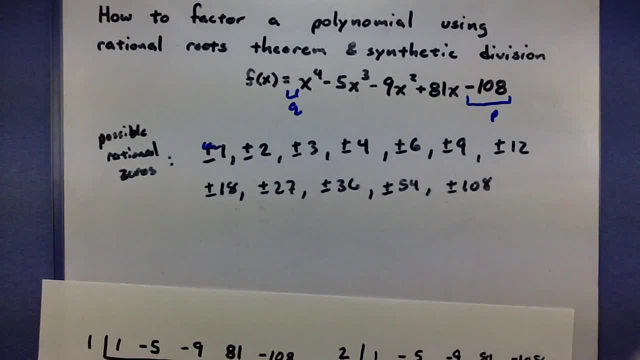 we found one And also go back to my list and say, okay, well, it looks like the positive two didn't work, but the three did. Now we don't necessarily want to keep going on to the four, because the only way we cross something off the list is if something doesn't work. 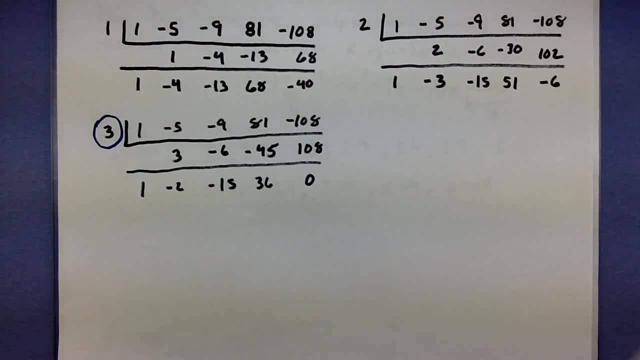 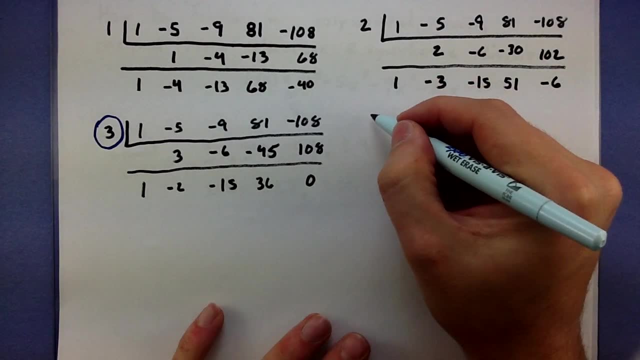 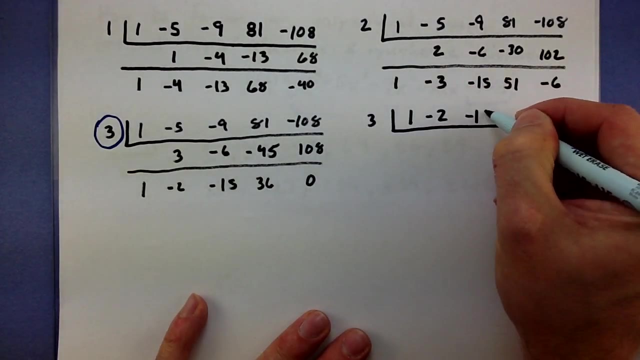 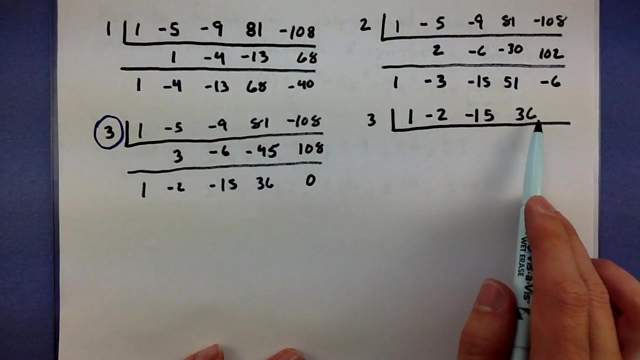 So if I know that three works, I'm actually going to try it again, and I'm going to try it in the reduced numbers down here Now. also, when looking at the reduced polynomial for here, notice how that my term is now 36 on the end. This means that I don't have 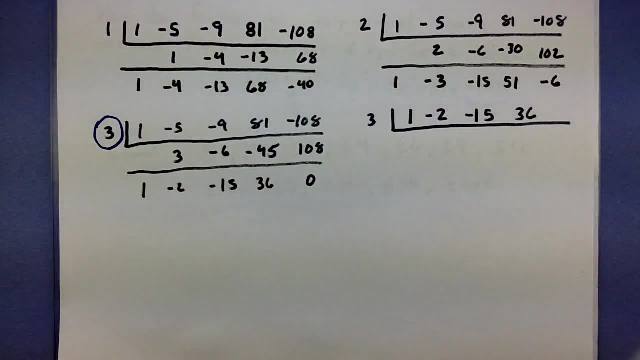 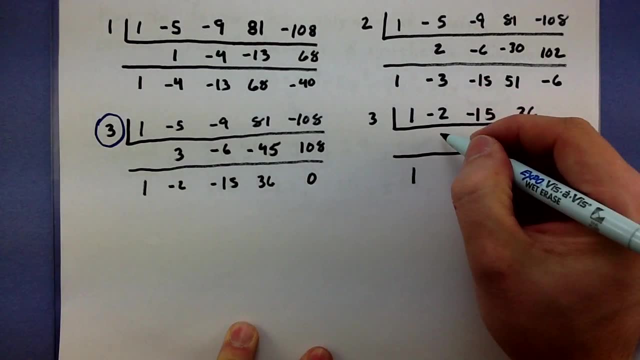 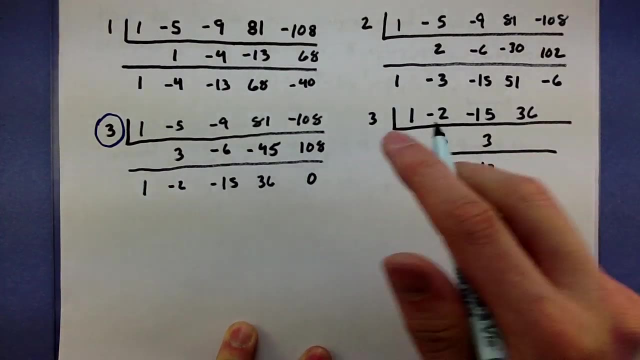 quite as many factors to consider as I did the first time. Anyway, let's go ahead and test out the three and give it a shot. So let's see: Drop it down, Multiply, Add, Multiply, Add And multiply. What do you know? It looks like the three worked again. 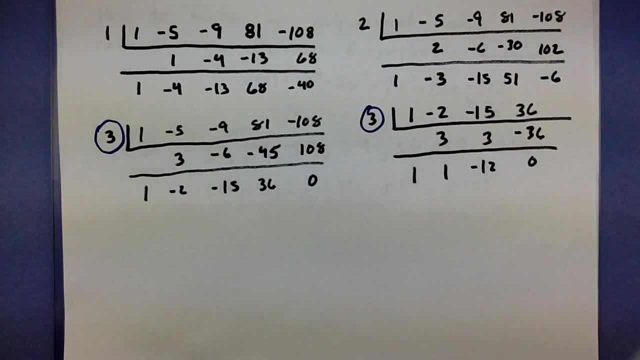 Let's keep it. And now look at our reduced polynomial. You always want to kind of keep an eye on this polynomial as you do find your zeros, because it gets smaller when you do find some of the factors, For example when we start at the very. 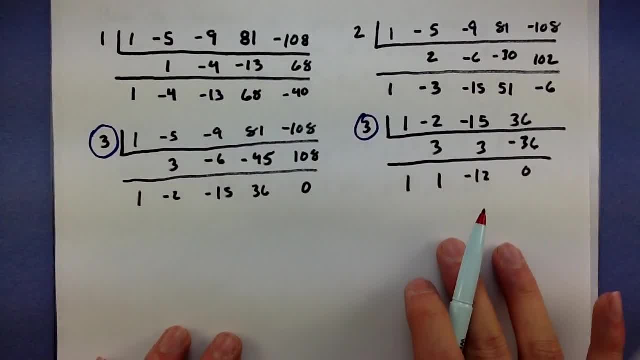 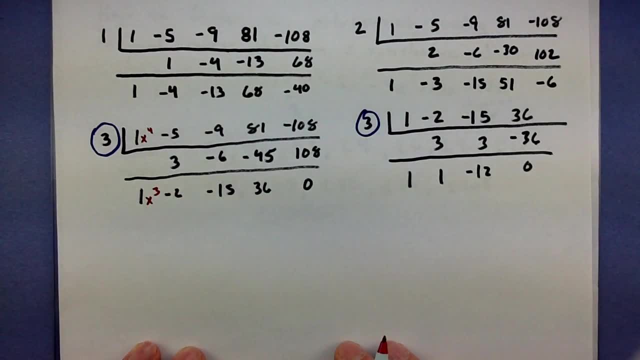 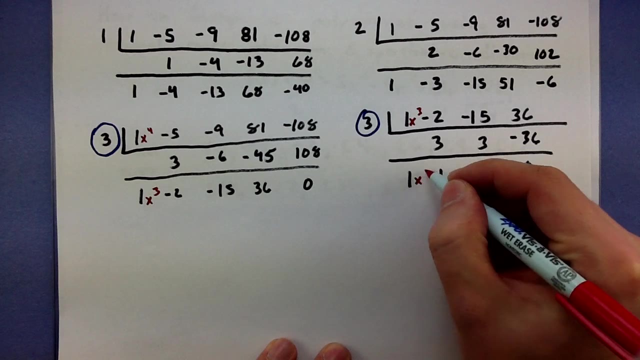 beginning we had an x to the fourth, So this is like a little x to the fourth here. But when we found this first zero, we reduced it to an x cubed. Then we used that reduced polynomial and we found another zero. so now this is an x squared. 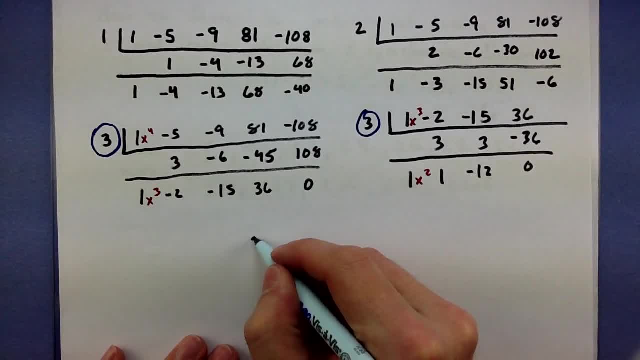 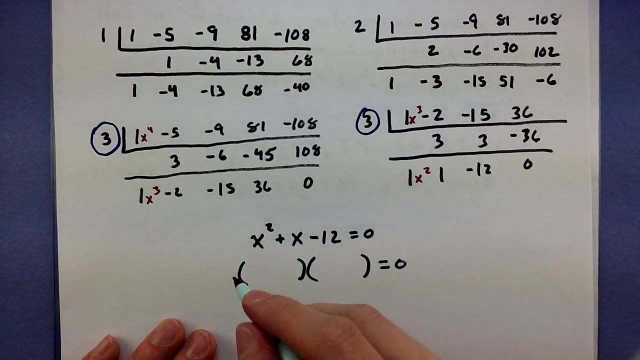 Now what that tells me, as soon as I get down to an x squared, is that maybe I can just factor this and find my last two zeros. And sure enough, it looks like this guy does factor. Let's see, This will factor into. 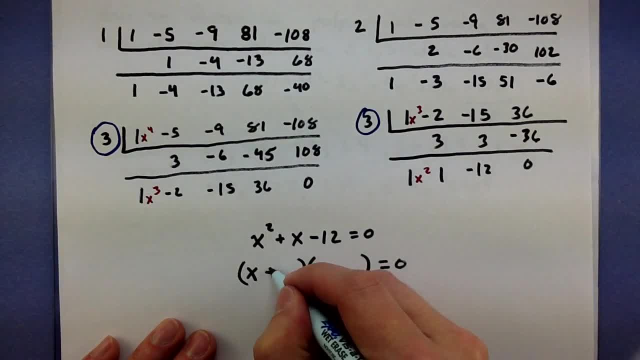 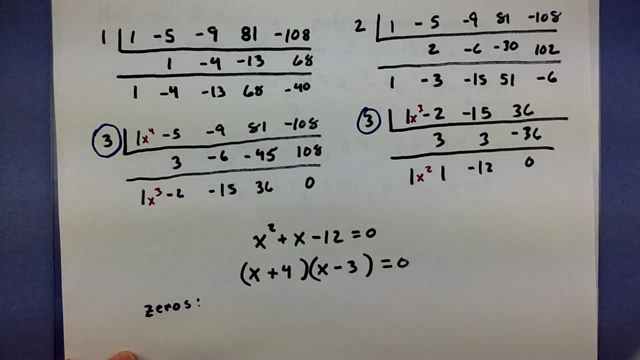 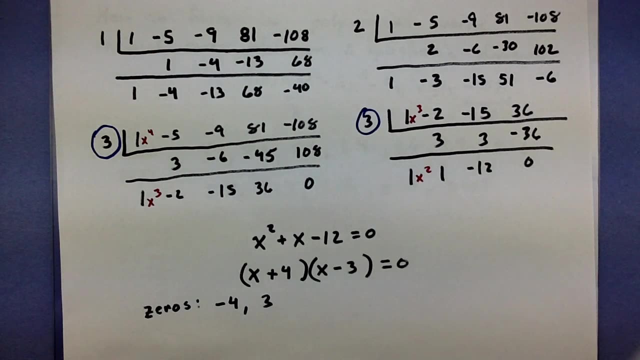 x And I got a plus four and a minus three, Which means my last two zeros. I have a minus four. It looks like three again. Well, notice how this fits pretty good with my possibilities. I have one, two, three positive zeros and one negative. 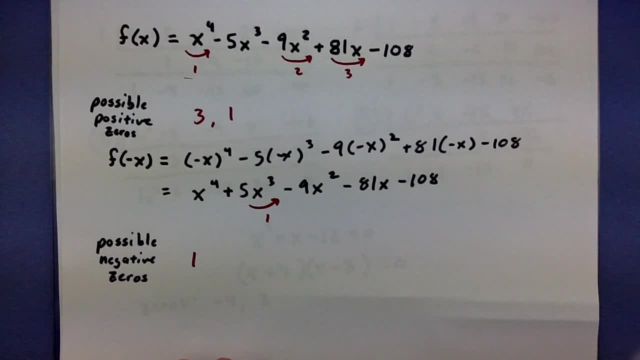 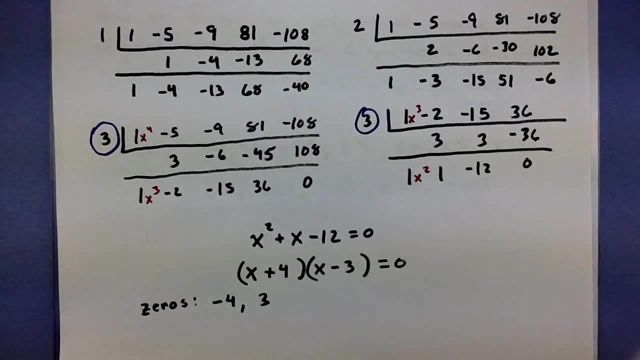 That's one of the possibilities. Descartes' rule of science said we'd come across That three of them are positive and one is negative. So alright, we know we're on the right track here. Let's go ahead and list out all. 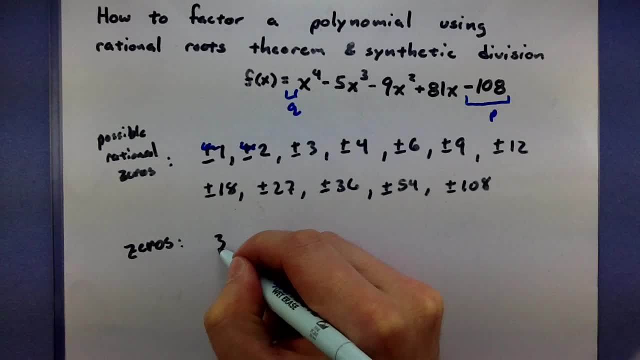 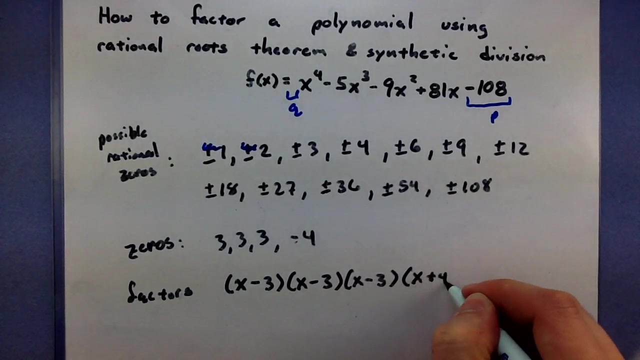 the zeros we found And from these we want to build the factors. The factors are always x minus the zero. So I have x minus three, x minus three, x minus three and x plus four. Well, really, since all of these are the same,